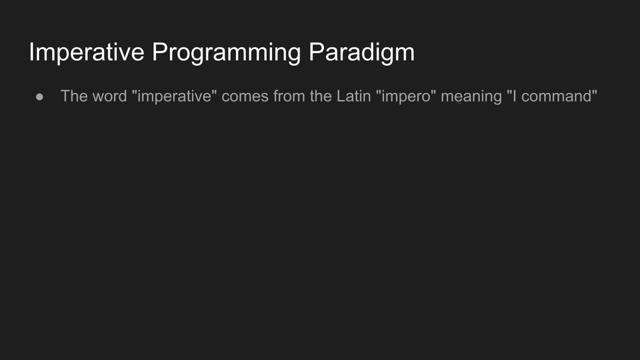 try to multiply two numbers, try to divide two numbers like that. Here these are the commands. So this is the first definition. Second definition is imperative. programming is a paradigm of computer programming in which the program describes the sequence of steps that change the state of the computer. So let us consider a scenario, If suppose, if you want. 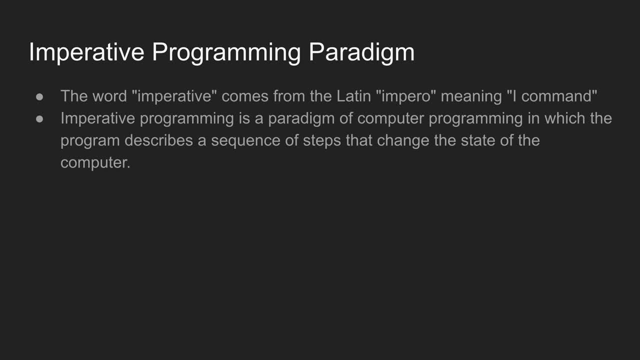 to add two numbers. you need to communicate that instruction to this system in such a way that machine can understand in. a machine can understand easily. So our task is to add two numbers. So for what you will do, try to do, is you will try to communicate with the machine. So this is your we. 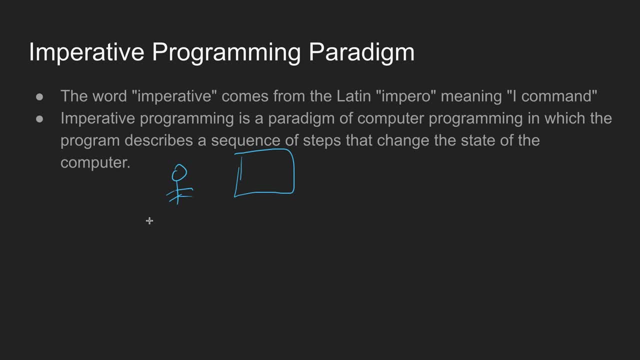 can say: this is yourself and this is called system. The first step would be get two numbers from the users, So get two numbers. and the second step would be- second command would be: add those two numbers. add two numbers. This is the second command. Third command would be display the. 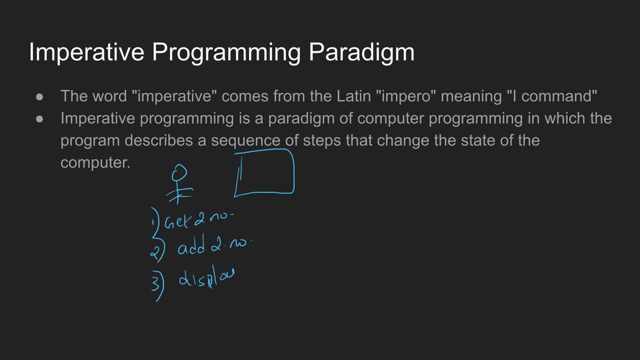 output display the sum display: sum. So these are the three commands. We will try to come, we will try to command, we will try to tell the machine with these three commands which will execute this commands in a better manner. So this is the second step. 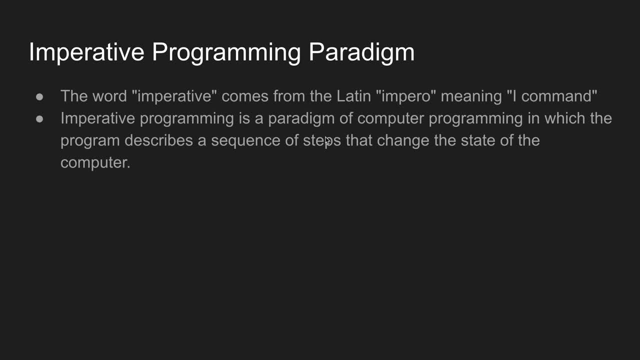 Imperative programming is a paradigm of computer programming in which the program describes a sequence of steps that changes the state of the computer. And the third point is it tells the computer how to accomplish this task. This is the important point Here. we are trying to tell the machine that you try to do this work in a this way, so that that 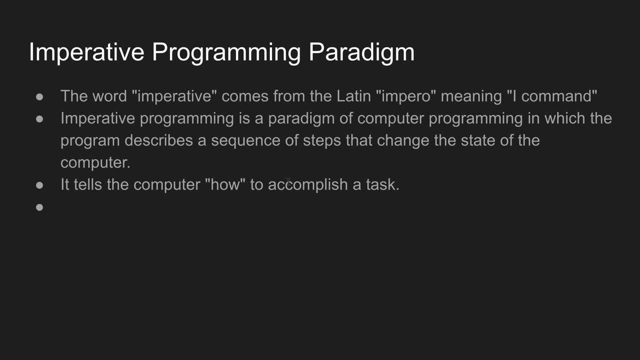 would be in a that would be executed in a better way. So we are trying to guide the mission. that's the important point: how to accomplish a task. And then programs returns with. programs written with this way often compile to binary acceptable code that runs more efficiently since all CPU. 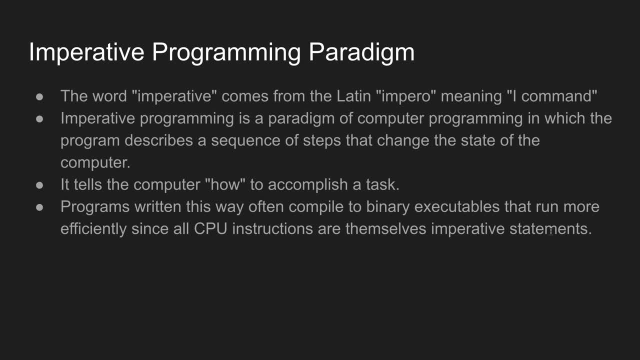 instructions are themselves imperative statements. So we will try to relate this with the real world examples. So, for example, if suppose if you want to run the CPU fan, then there could be some statement which could be called as imperative statements. If suppose, if you want to switch on or switch off the